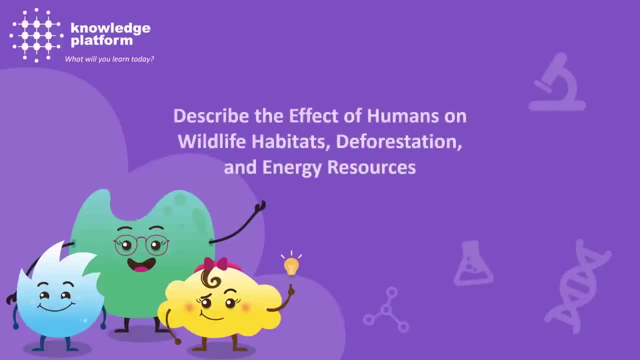 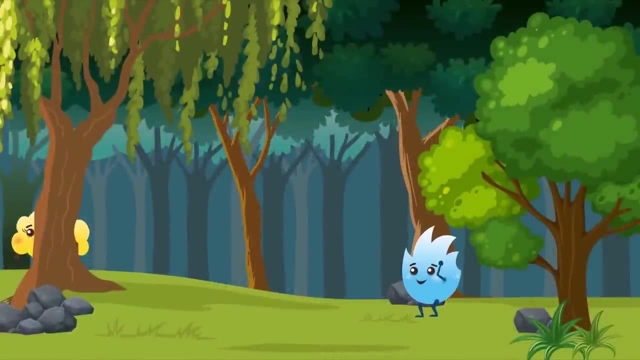 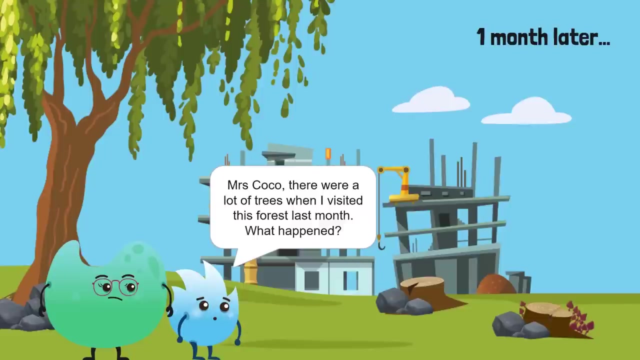 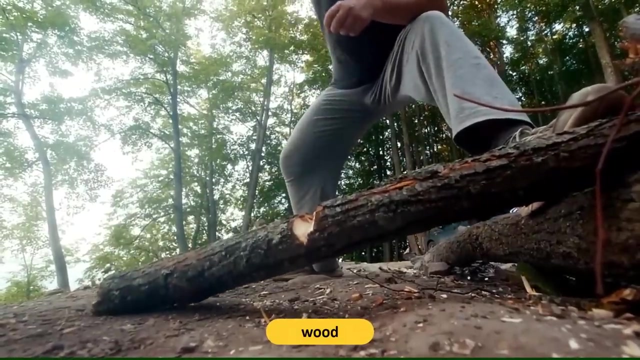 Mrs Coco, there were a lot of trees when I visited this forest last month. What happened, Spiky? they were cut down. There are many reasons why people cut down trees. They cut them for wood or to clear the land for construction of houses and buildings. 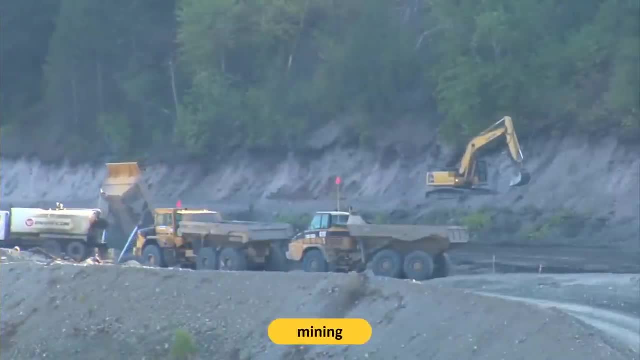 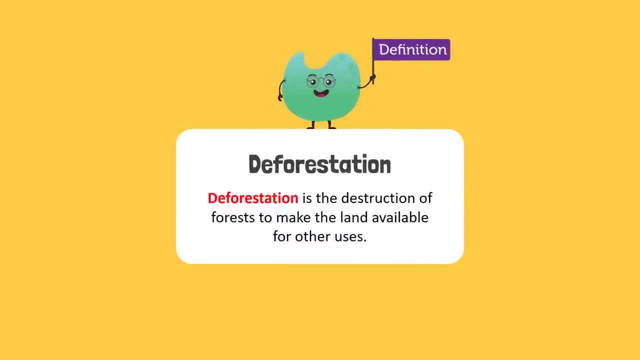 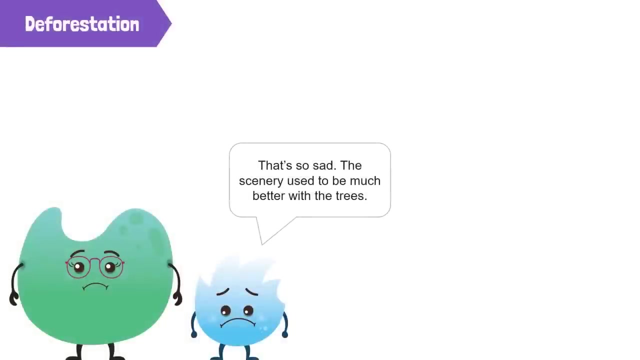 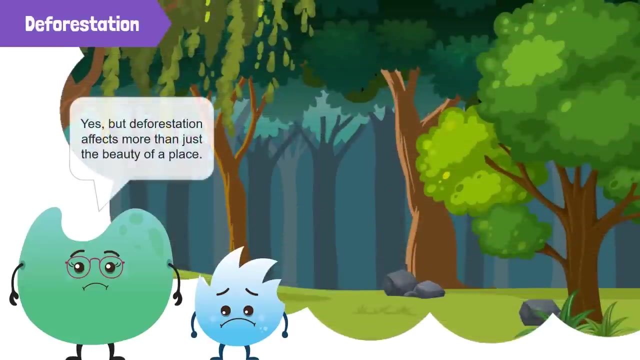 Sometimes forests are cleared for mining as well. This is known as deforestation. Deforestation is the destruction of forests to make the land available for other uses. That's so sad. The scenery used to be much better with the trees, Yes, but deforestation affects more than just the beauty of a place. It also has a negative impact on the environment. 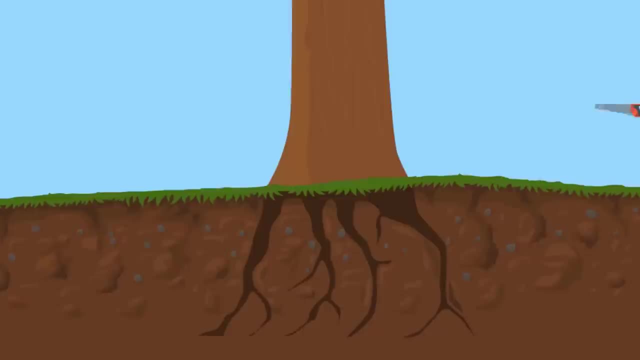 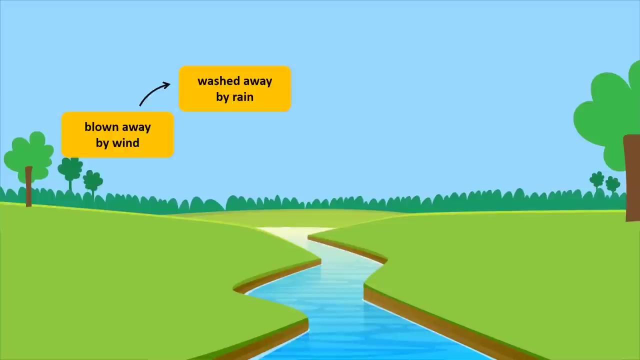 The roots of the trees hold the soil together. When we remove the trees, the soil is exposed and often blown away by the wind. The soil is washed away by rain. The eroded soil is deposited in rivers and streams, blocking the flow of water. 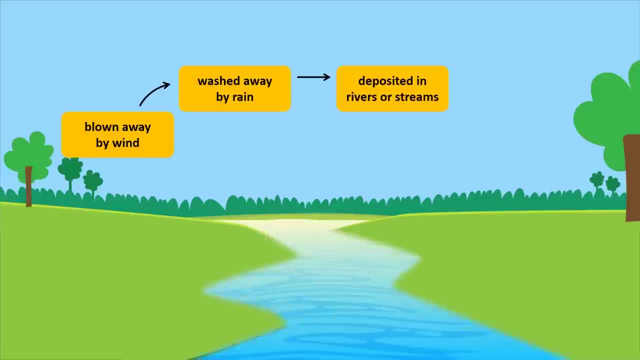 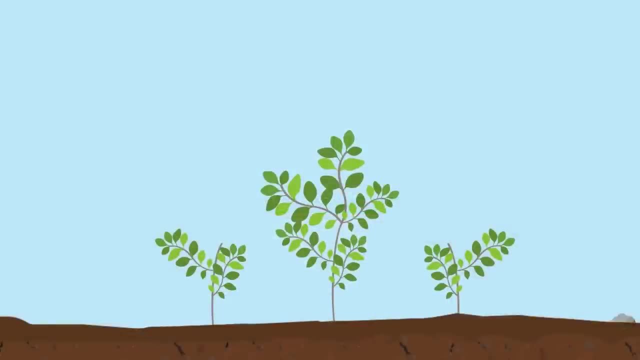 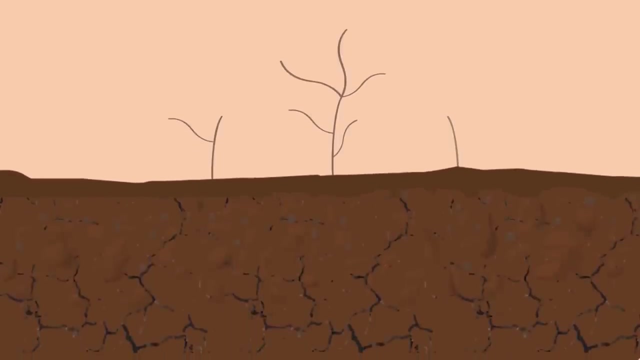 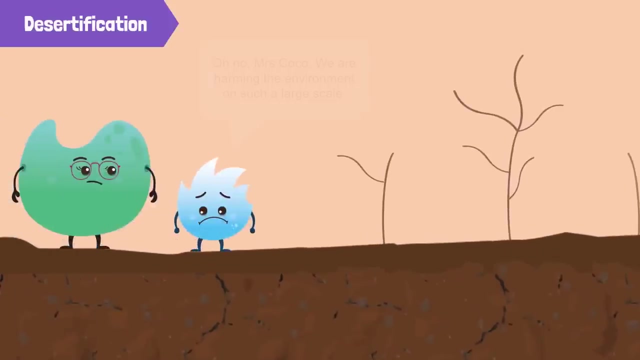 The water level in the rivers then rises rapidly, causing floods. Also, when this topsoil erodes, plant growth becomes impossible and the land becomes barren like a desert. This is known as desertification. Oh no, Mrs Coco, We are harming the environment on such a large scale. 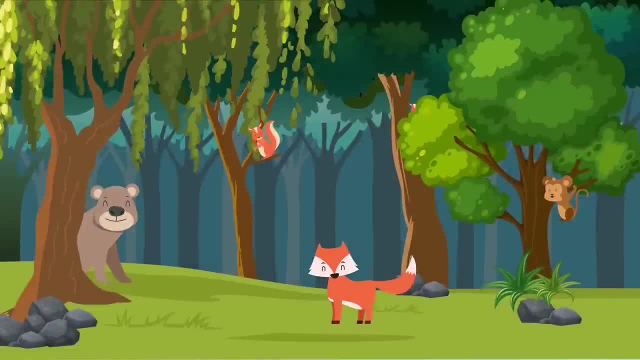 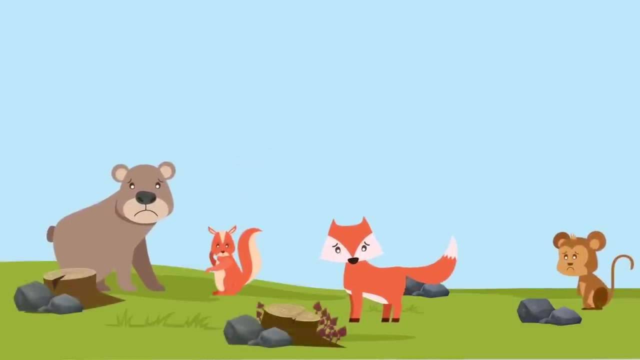 Not only the environment, Spiky, We are also harming the wildlife. This includes wild plants and animals. When we cut trees down, we are leaving less space for animals to live. This is known as desertification. Think about all the animals that live in forests. Where would they go if we destroy those forests? 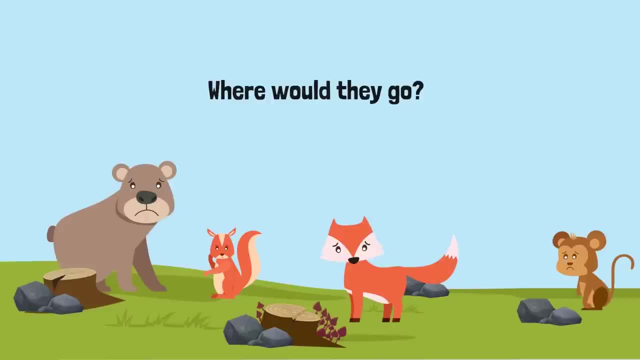 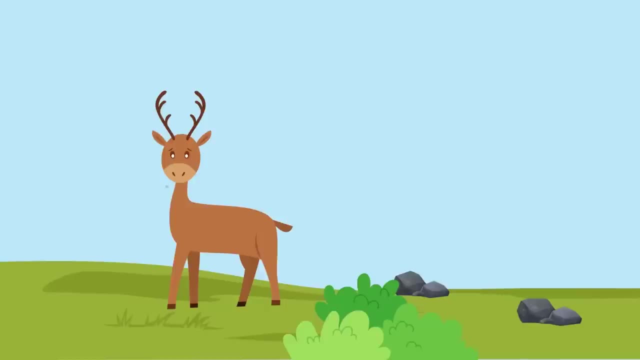 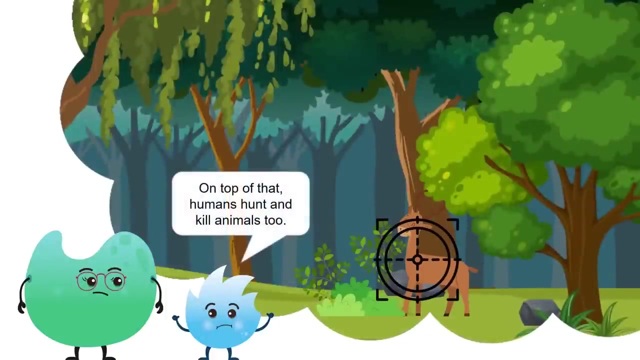 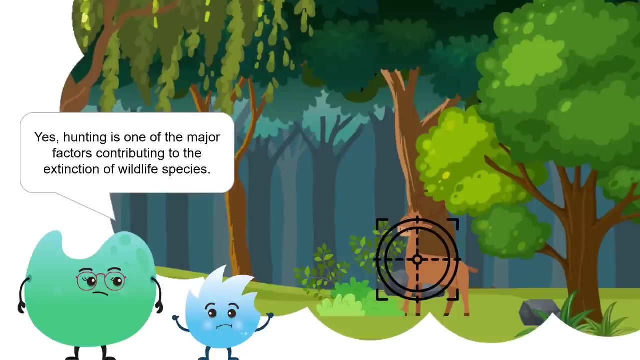 We are destroying their homes. Also, animals that eat plants for food. what would they eat? As a result, many animals do not survive and sometimes they even go extinct. On top of that, humans hunt and kill animals too. Yes, hunting is one of the major factors contributing to the extinction of wildlife species. 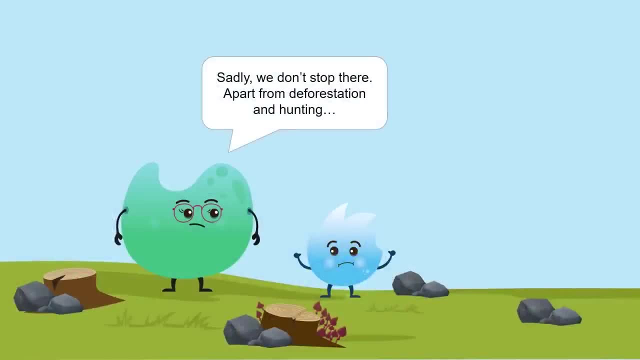 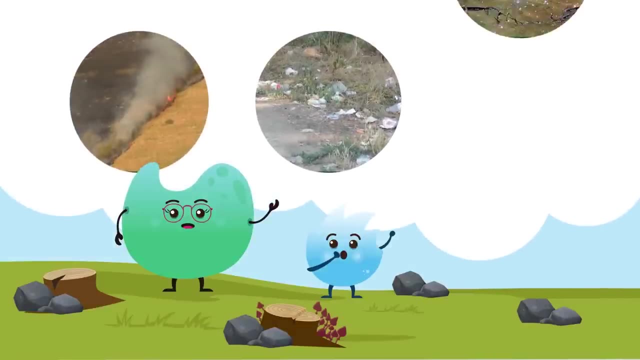 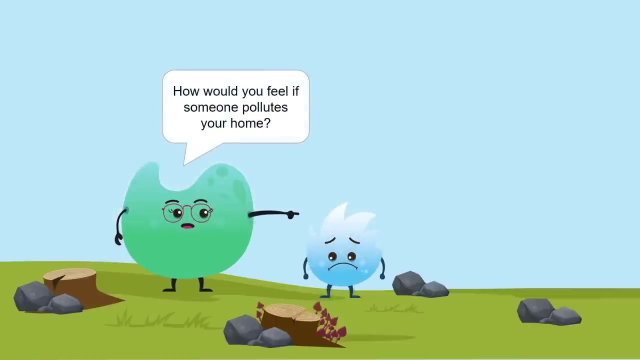 Sadly, we don't stop there. Apart from deforestation and hunting, we have polluted the air, land and water. How would you feel if someone pollutes your home? You might end up being sick. This is what humans are doing to animals and their habitats, Spiky. 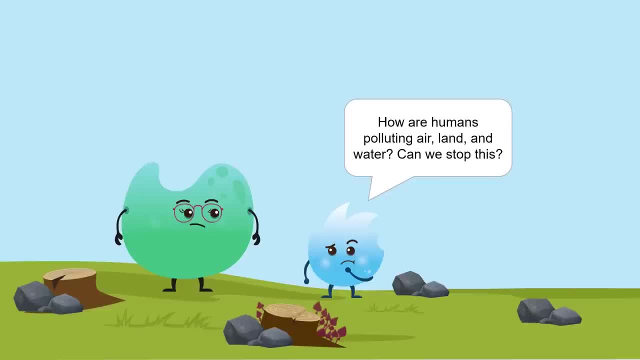 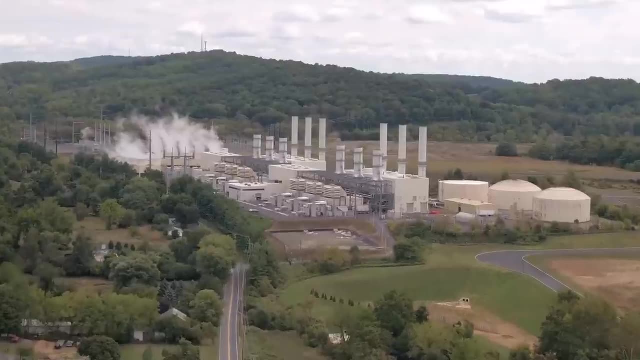 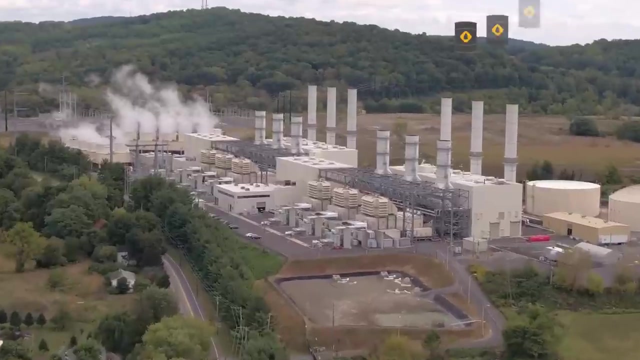 This is so sad, Mrs Coco. How are humans polluting air, land and water? Can we stop this? The major sources of pollution are industrial processes and electricity generation. We are burning millions of barrels of fuel every day. The burning of fossil fuels produces a lot of pollution. 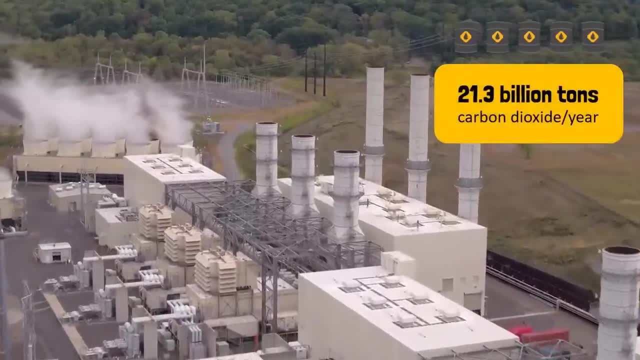 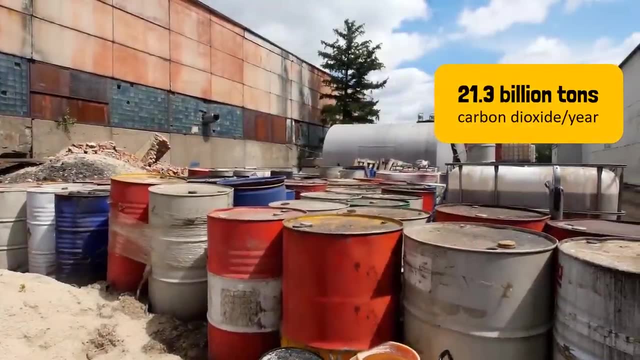 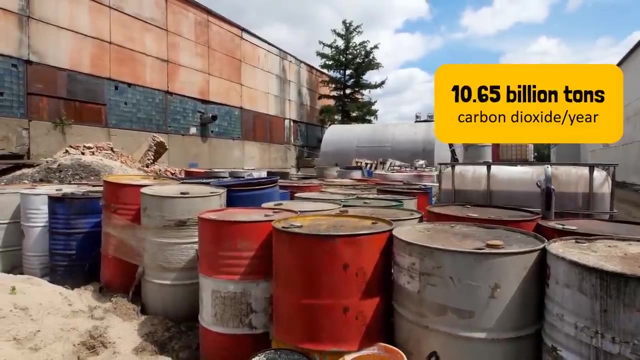 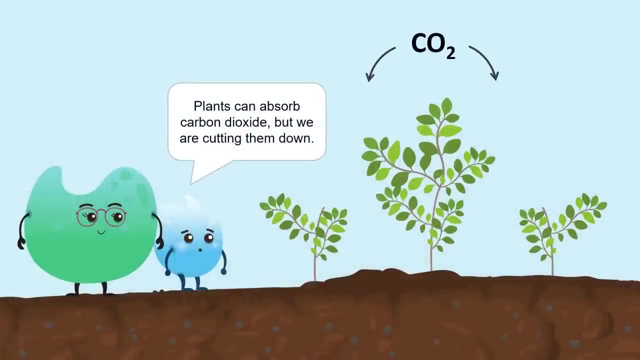 It produces 21.3 billion tonnes of carbon dioxide per year. It is estimated that natural processes can only absorb about half of that amount, So there is an increase of 10.65 billion tonnes of atmospheric carbon dioxide per year. Plants can absorb carbon dioxide, but we are cutting them down. 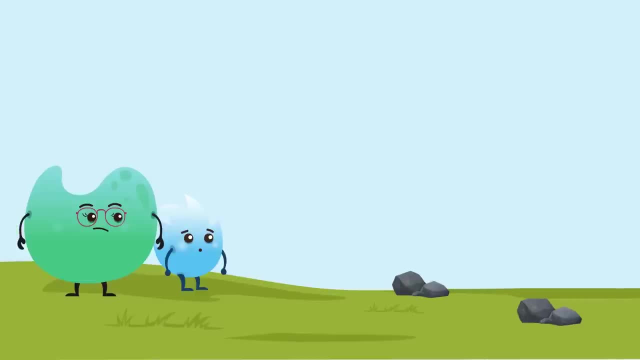 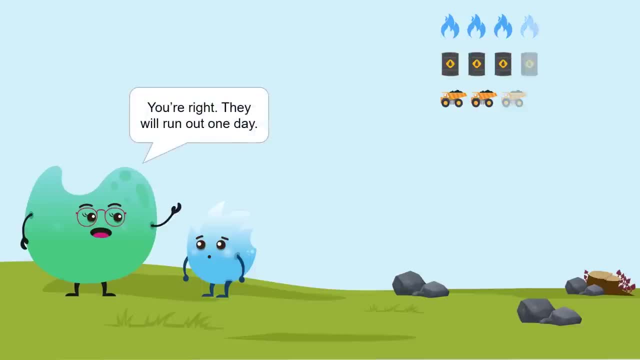 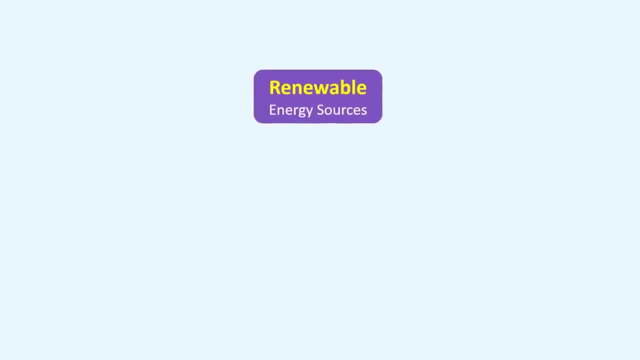 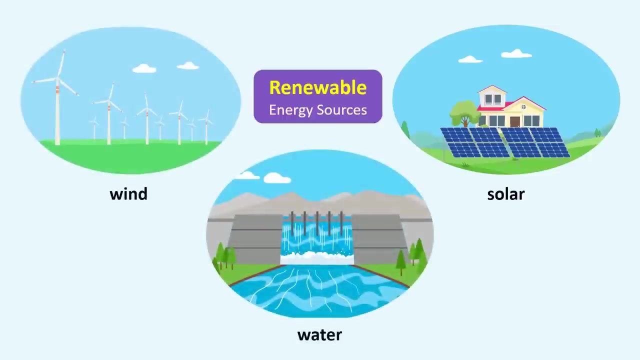 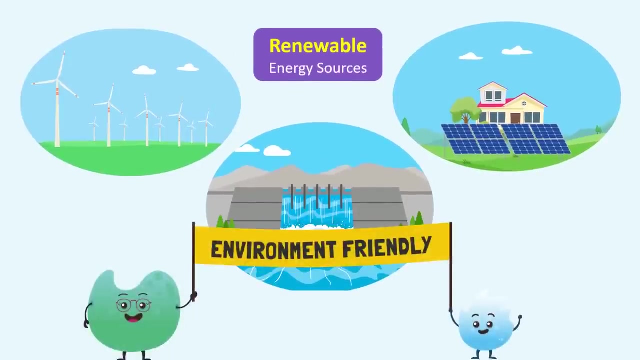 You're right: They will run out one day, Which is why we should try shifting to renewable energy sources such as solar, wind and water, to preserve fossil fuels as well as our environment. Also, renewable energy sources are environmentally friendly and don't cause pollution.